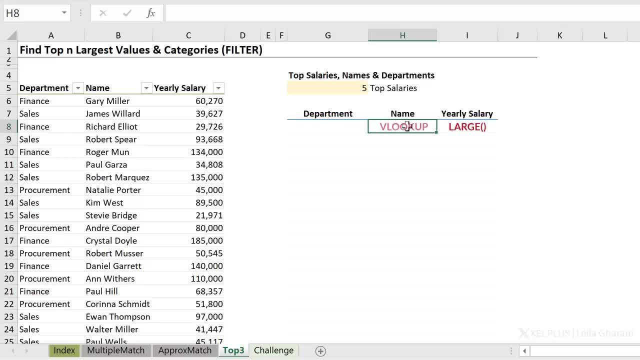 to get the salaries out, and then I was using VLOOKUP or INDEX AND MATCH to get the name of the person who earns this number. so basically my lookup value was the salary. I would have a problem, right, Because it's always going to find the first match. 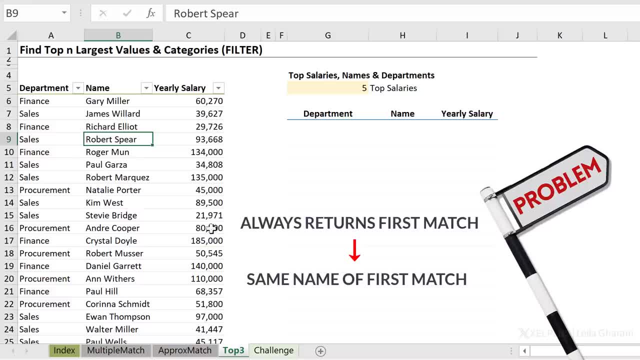 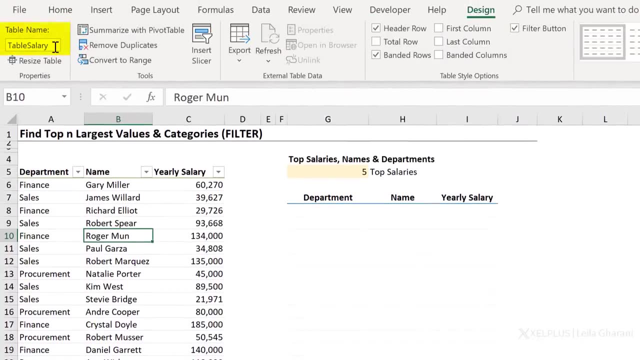 and it would always return the same name, even if there are other people earning that same salary here. But I wouldn't have this problem if I use the filter function correctly. The data in this table has been formatted as an official Excel tables under design. 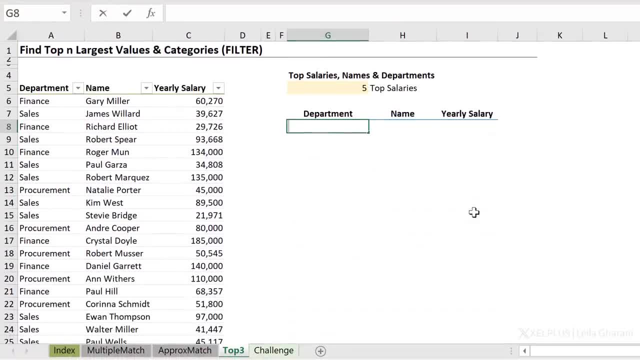 I've called it table salary. Now let's start using the filter function and seeing how we can tweak this to get what we want in a dynamic way. Array is the full table, because I want everything returned, So I'm going to hover to the side. 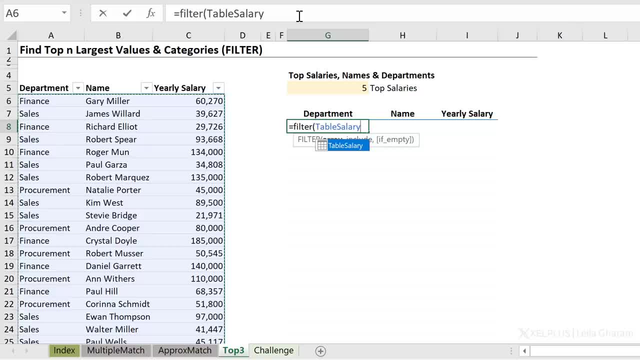 until I get that tilted arrow, click on it to include the table name in the formula. Next argument is the include argument. Basically, the driver of this is the salary right, So I want to include all salaries that fall in the top five. 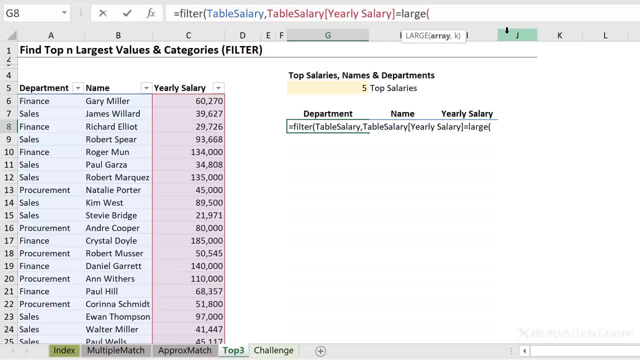 If I was going to say equals to find the fifth largest numbers, I would use the large function. my array would be this: my K would be this: close the bracket. This is just going to return the name of the person that earns the fifth largest salary. 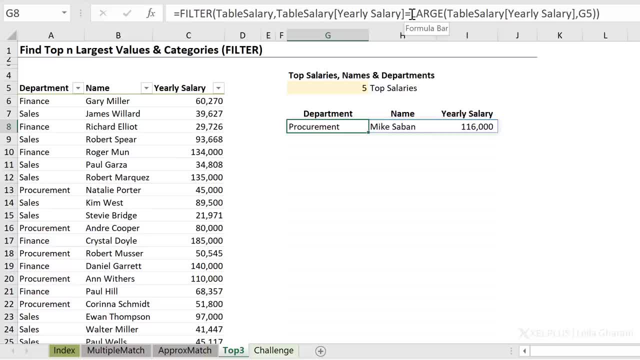 But how do I include the other ones, The first, second, third and fourth ones? Well, the easiest method to handle this is not to look for exactly the fifth largest salary, but instead to look for anything that's greater than or equal to the fifth largest salary. 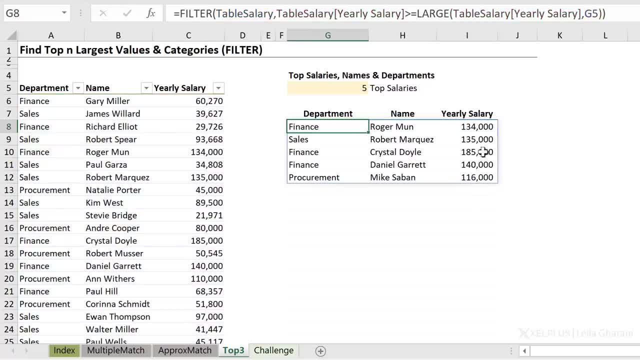 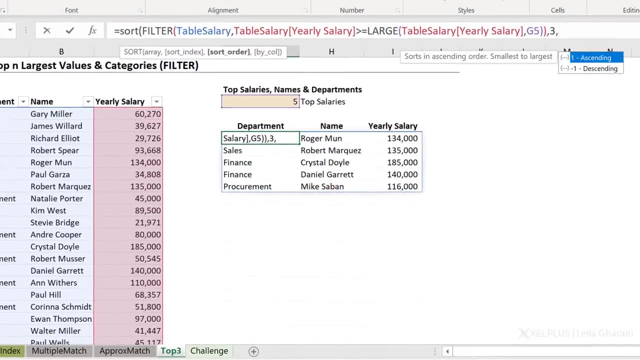 When I press enter I get my values. Now notice they aren't sorted. So to sort them by salary I can include the filter function inside the sort function. My sort index is the third columns. I have to put three and I want it in descending order, not ascending. 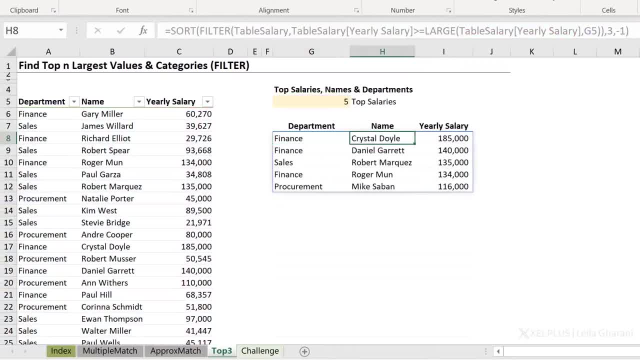 So I can put three and I want it in descending order, not ascending. So I can put three and I want it in descending order, not ascending, So minus one. Crystal Doyle from finance is earning the highest salary. then is Daniel from finance. 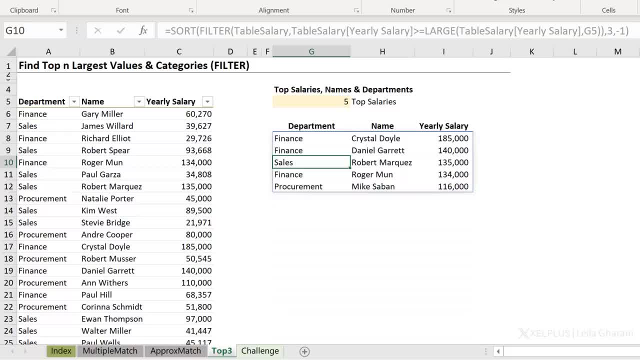 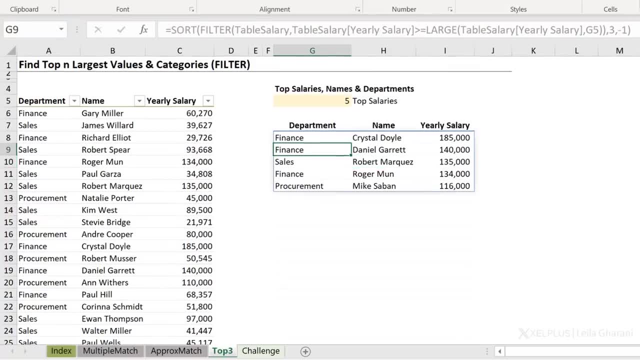 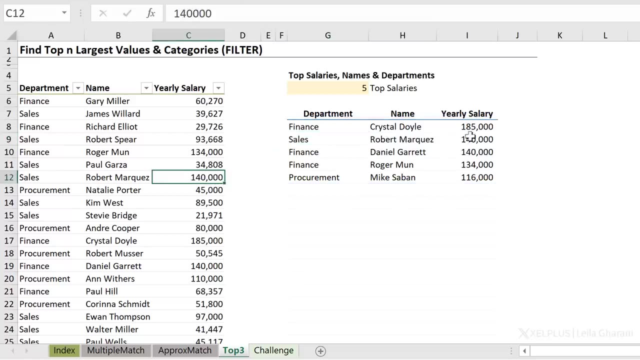 and then is Robert from sales and so on. Now let's just give them two identical salaries. So let's say Robert from sales department is going to get what Daniel gets from the finance department- 140,000,. the names here update automatically. 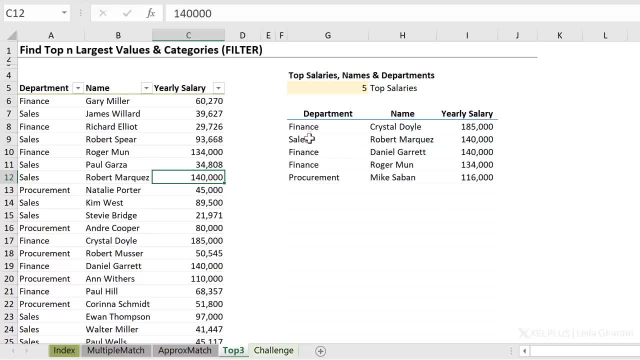 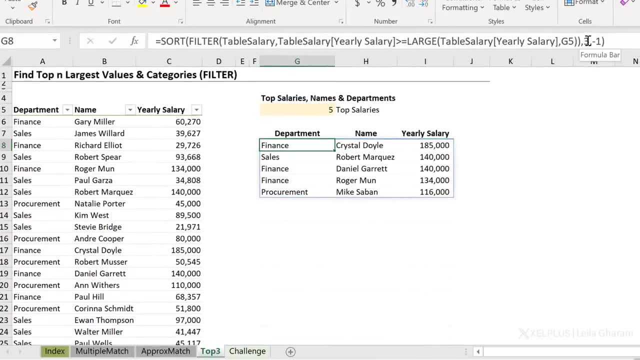 To sort this better I could add another level of sort right? So after this I could say sort by department Here I have to go and use my array constants For my sort index. I'm going to open the curly bracket. 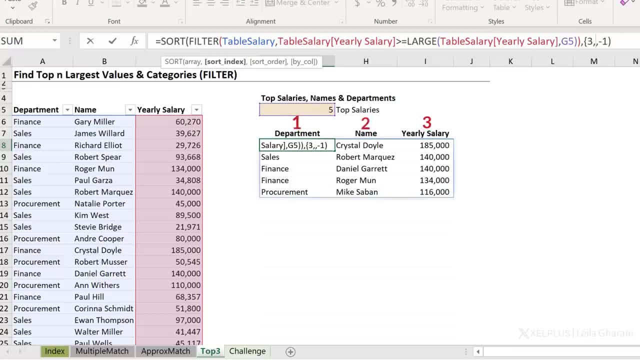 first sort by salary and then sort by department. Close the curly bracket. For my sort order I want to have yearly salary in descending order and department in ascending order. Close the curly bracket. This way I get four. I get finance here together. 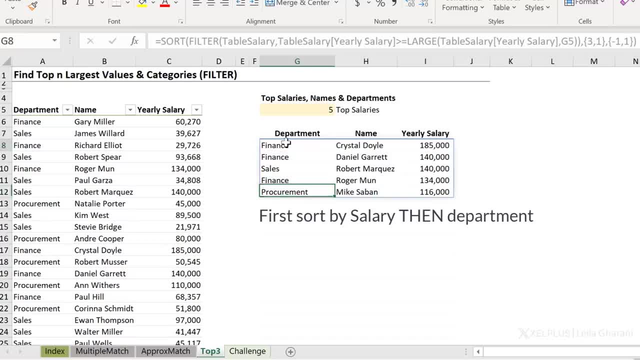 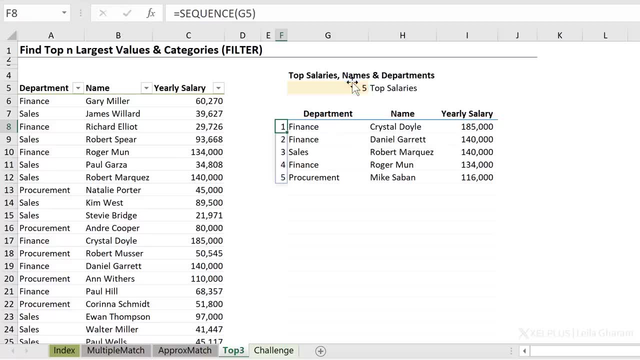 and then I get sales finance and so on. Okay, so now let's just improve this report by adding the sequence function here as well. There's one other thing we can do, because if we don't restrict this with the data validation, 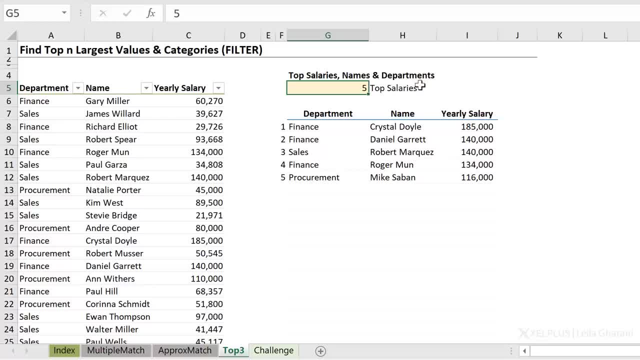 people could come in and input a really huge number like 100 or 200, and our data's going to spill. We could actually take care of that inside the formula as well. We can use an if here For our logical test. we're going to count. 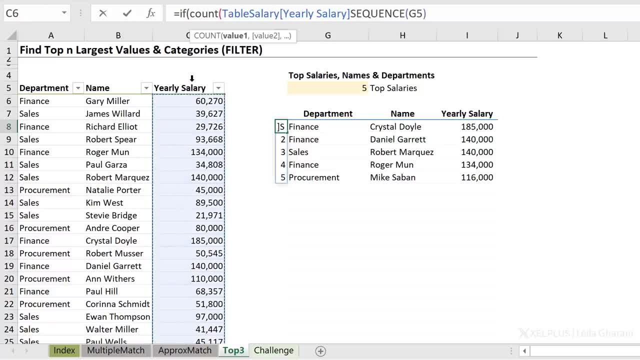 the number of values we have in here, and if this is greater than the number that we input here, we're going to run our sequence, but if it's not, we're going to give some message to the user: report too large and close the bracket. 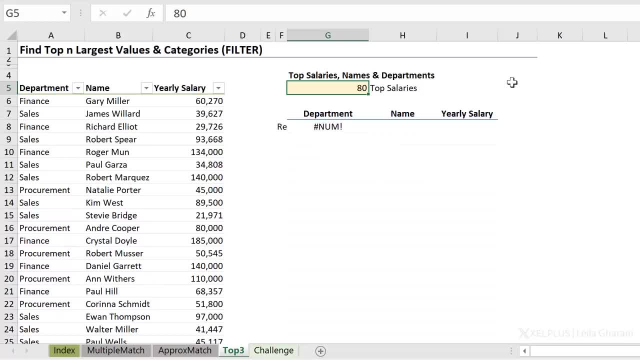 So let's just test this. What if I put 18 here and press enter? I get here report too large and here I get an error, because my large formula is going to end up returning errors. It's not going to find the 80th largest salary in here. 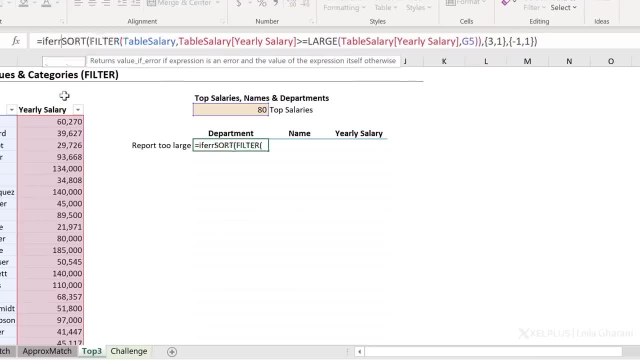 because it doesn't exist. So in case I run into an error, I can use if error and then put something like: please input smaller number, Okay. so whatever message you want to give you can include in here, but this also takes care.